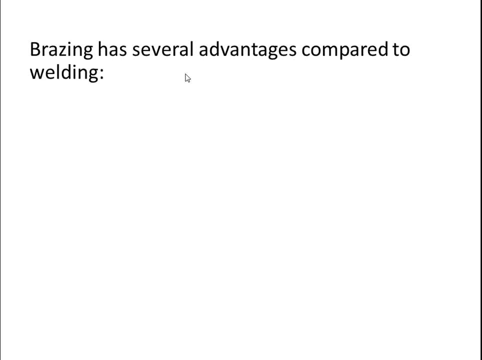 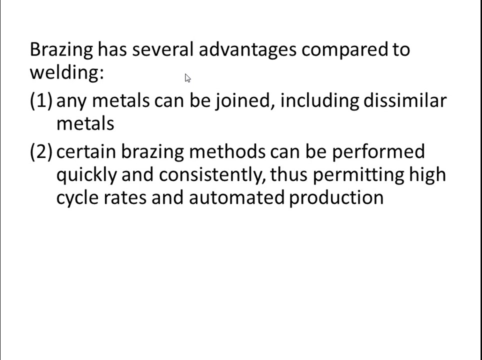 Brazing has several advantages compared to welding. The first one is any metals can be joined, including dissimilar metals. Second one: certain brazing methods can be performed quickly and consistently, thus permitting high cycle rates and automated production. Third one: some methods allow multiple joints to be brazed simultaneously. 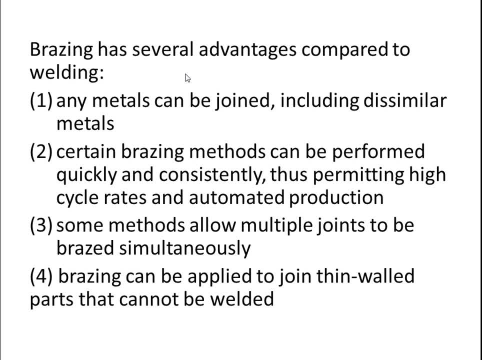 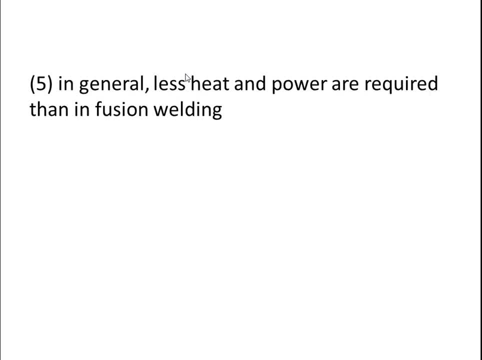 Four brazing can be applied to join thin wall parts that cannot be welded. Fifth: in general less heat and power are required than in fusion welding. Six problems with the heat affected zone can be solved. Problems with the heat affected zone in the base metal near the joint are reduced. 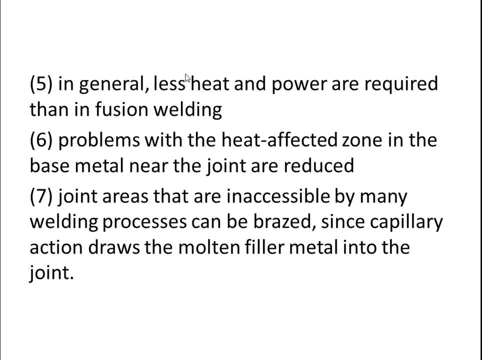 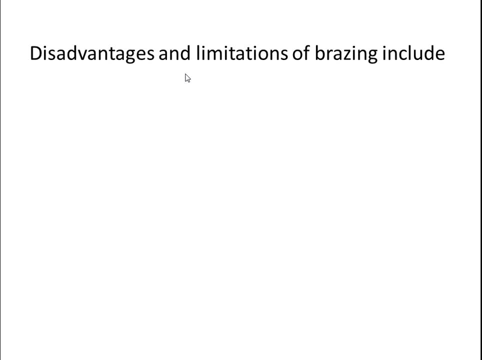 Seven joint areas that are inaccessible by many welding processes can be brazed, since capillary action draws the molten filler metal into the joint. And there are some disadvantages and limitations of brazing include, First one: joint strength is generally less than that of a welding joint. 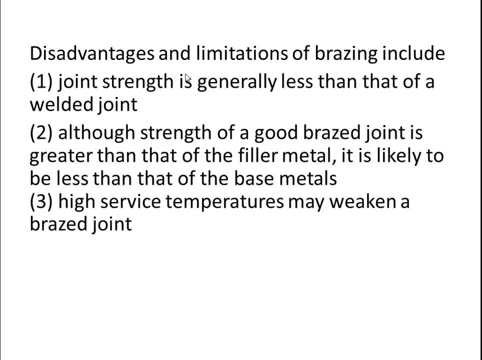 Second, although strength of a good brazed joint is greater than that of the filler metal, it is likely to be less than that of the base metals. Third, high service temperatures may weaken a brazed joint. Fourth, the color of the metal in the brazed joint may not match the color of the base metal parts, a possible aesthetic disadvantage. 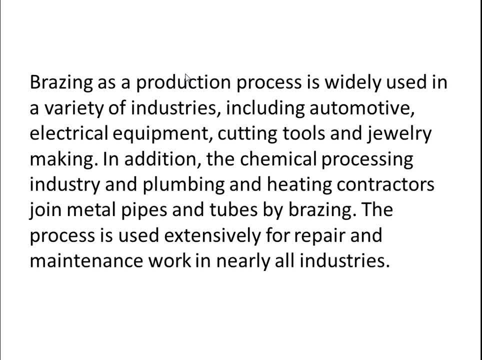 Brazing as a production process is widely used in a variety of industries, including automotive, electrical equipment, cutting tools and jewelry making. In addition, the chemical processing industry and plumbing and heating contractors join metal pipes and tubes by brazing. The process is used extensively for repair and maintenance work in nearly all industries. 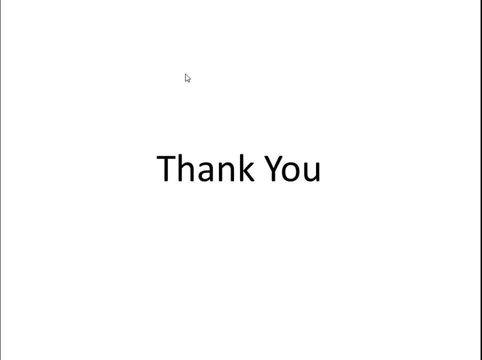 And finally, thank you for being with me.